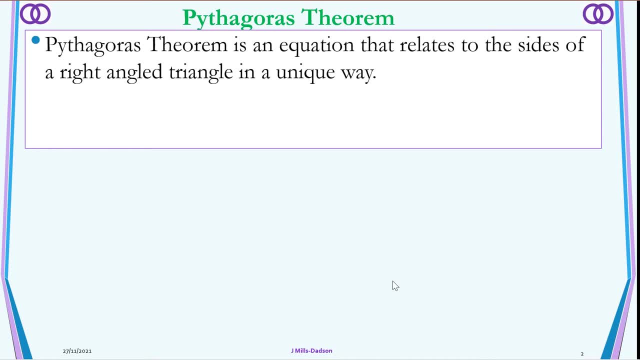 Now, Pythagoras Theorem is an equation that relates to the sides of right angle triangle in a very unique way. What it says is this: the square of the longest side, normally called the hypotenuse. this is the longest side. the side facing the right angle is the hypotenuse, so the square on this hypotenuse is equal to the sum of squares of the other two sides. 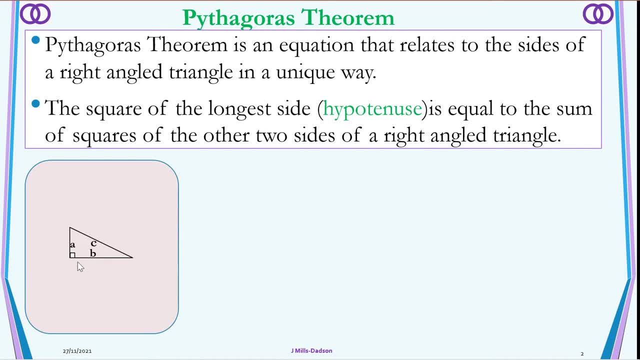 Now, the square on side A and the square on side B together must be equal to the square on side C. In short, this is what the theorem is all about. So, using diagrams, if this side is A square, on side A, the area will be A squared, because A times A is A squared. 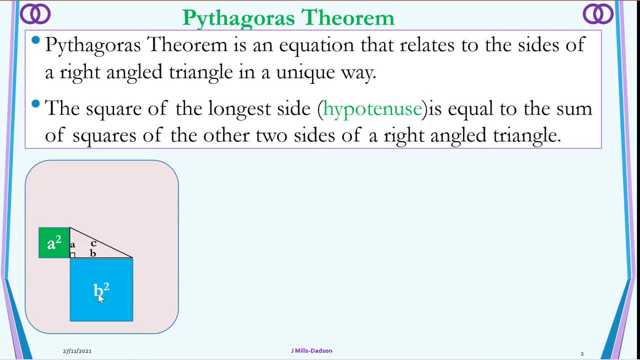 Then on B, the side B, the area will be B squared. So we are saying that A squared and B squared should equal to the square on side A. Now the square on side C, Let's see. So. to prove that I can make an area of A squared and B squared equal to C squared, I'm going to divide B squared into four identical right angle triangles. 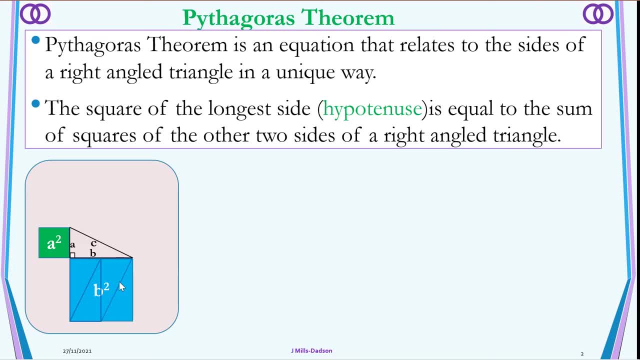 And I'm going to rearrange the four identical right angle triangles in the green to make a bigger square on C. So I'm going to move them one by one: First one, second one, the third And the last. So now I can now put in my little square there. 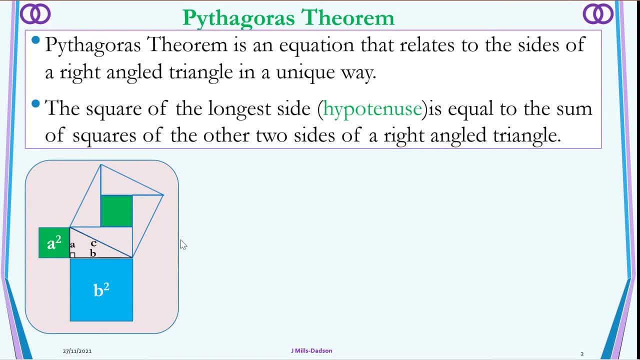 And it's true that this square represents C squared. As you can see, it represents C squared, So algebraically it means that C squared, the area is equal to A squared plus B squared. So that's what the theorem is all about. 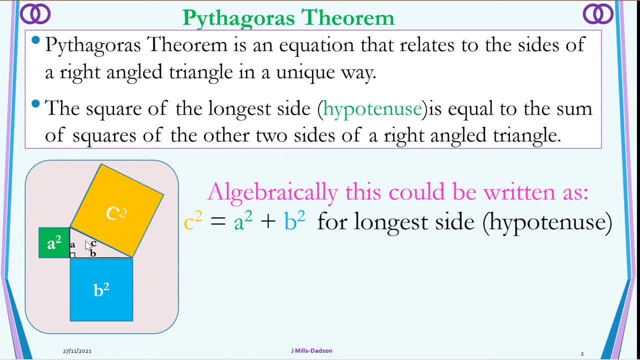 And this is normally used when you are looking for the logarithm- The longest side of the right angle triangle. If not, we use the subtraction rule for the other side. So if it is this side, it's C squared minus B squared to get A squared. 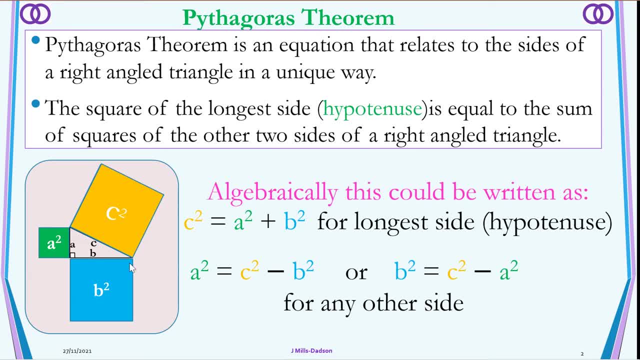 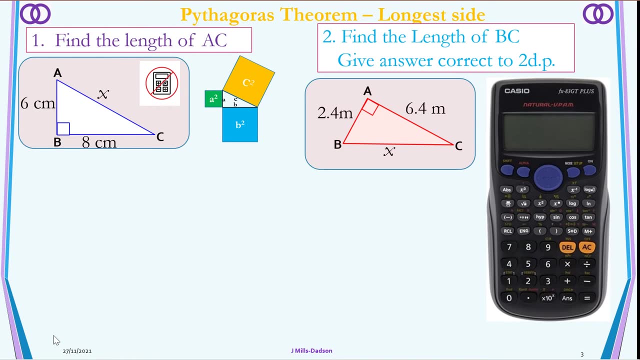 Or if it is this side, C squared minus A squared. So actually what matters is that longest side always use the addition rule And the other side subtraction rule. So let's look at a simple exam question. We have the non-calculator method where you have to go through step by step. 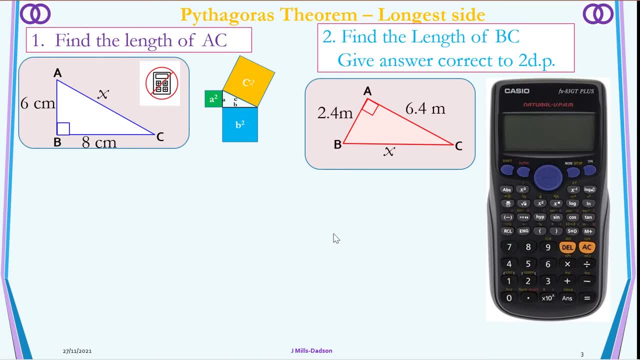 And the calculator method, where you have to quickly use the calculator to get the answer. So here we call your formula longest side. So it means I'm going to square this side and add this to this side. That's the relationship. 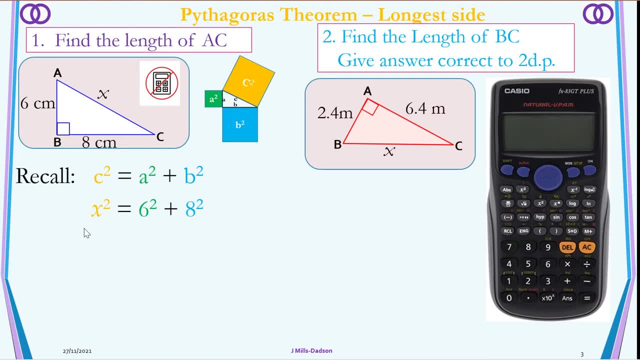 So X squared to replace C will be seen as 6 squared plus A squared. 6 squared means 6 times 6.. A squared A times 8.. So be careful about that Next line. work out these values. 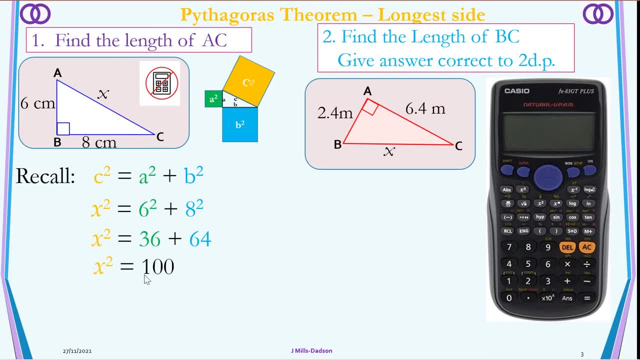 Next line: add these numbers. Next line we are looking for X and not X squared, So you need to work out square root on both sides And that will give you 10C. So X is 10C When it's calculator method. just remember, because at the end we're going to find the square root. 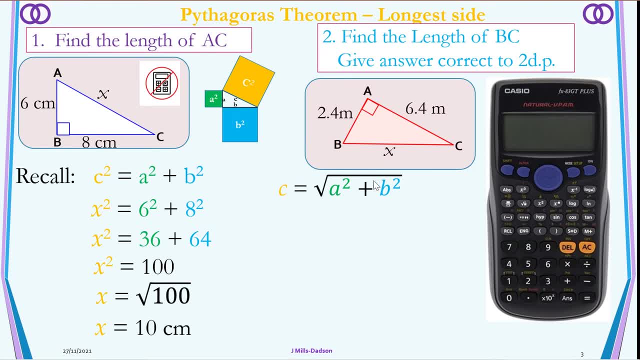 And it's an addition rule- You just have to start with the square root and just do exactly what you normally do, So you don't need to go through all these steps. So this is your A, This is your B Square, each of them and just put them under the square root. 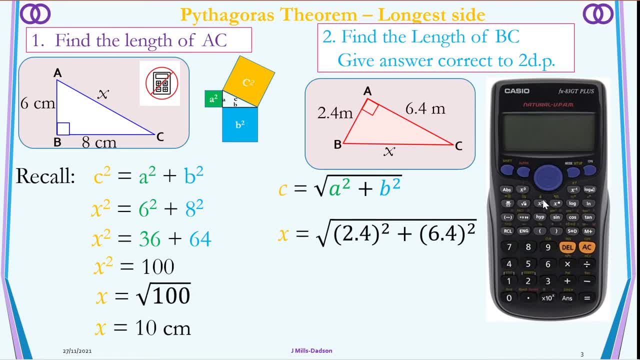 So you just hit the square root button 2.4.. The X squared represents square. You hit the X squared, the square will come Plus 6.4.. Hit the square button, the square will come. Then you press the equal sign. 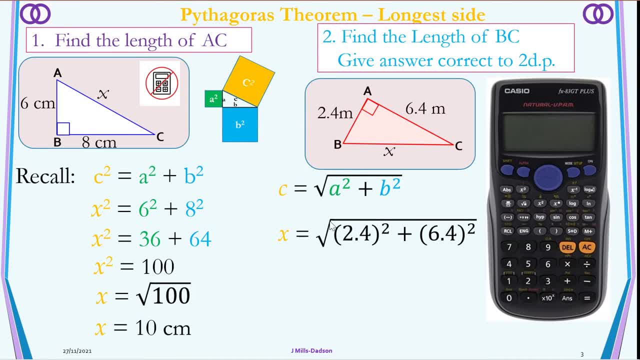 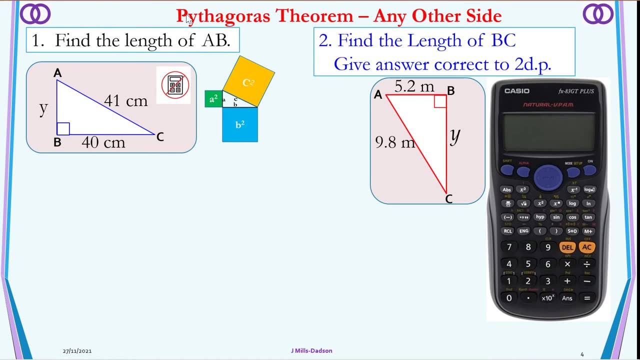 And that will give you the answer. Make sure, if you're using a bracket, close the bracket before you press the square button And you get your answer at 6. 6.84 meters when you approximate. Now let's look at what if it is not the longest side. 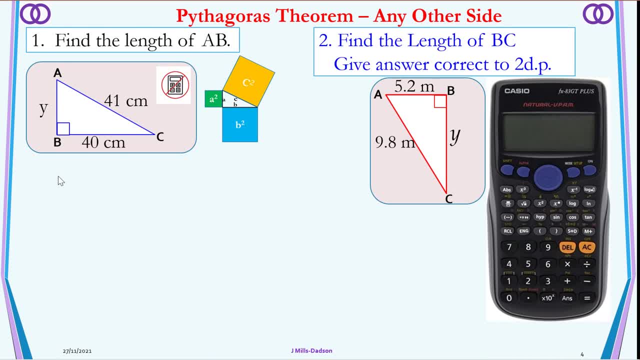 Now calculate the method the same way. So not the longest side is the fraction rule, So we start with the biggest number squared minus the other number squared, So Y squared will be equal to 41 squared minus 40 squared. 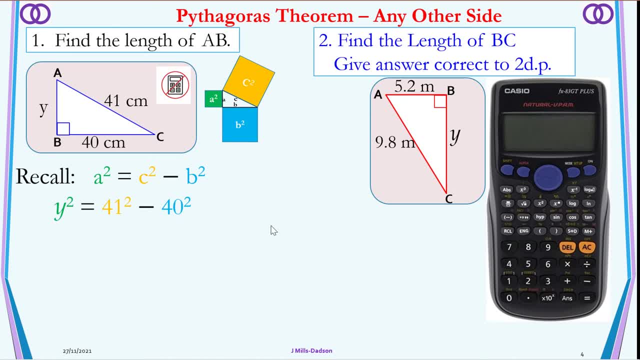 When it's non-calculator and the numbers are big, do side working by doing 41 times 41.. 40 times 40 to get your answers before you continue. so next line: work this out. next line: find square root on both side. the square root will cancel out the 2. 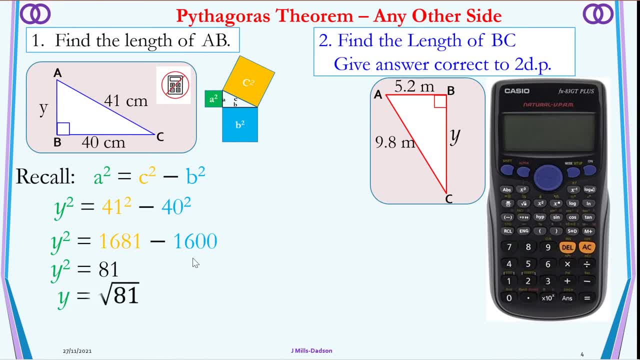 sorry the square. so Y square becomes Y and square root of 81. that gives you 9C calculator method. you check it's not a longer side, so it's subtraction rule. so you start with the square root of C squared minus B squared. so if you 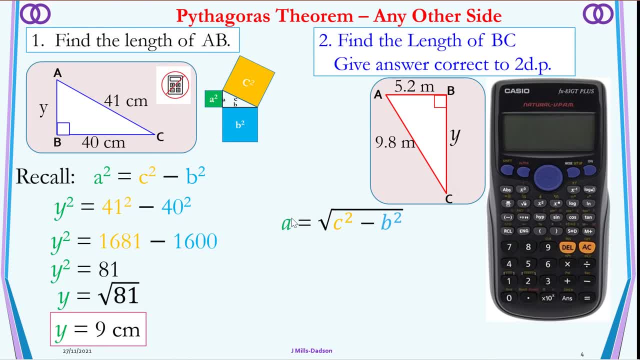 remember, when we're doing this calculator method, we don't start with a square, because we're taking care of it by using the square root sign straight away. when the calculator method we start with the square on to the final one, you find a square root. so know the difference. so the longer side first. nine: 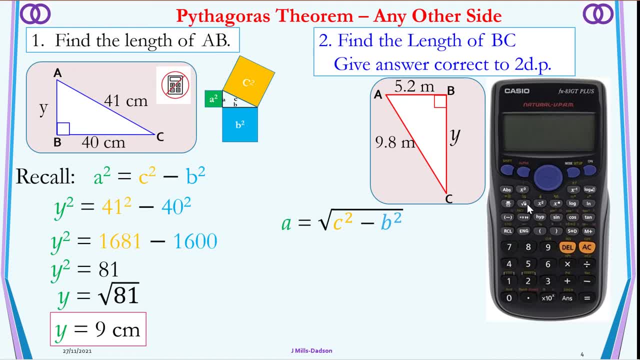 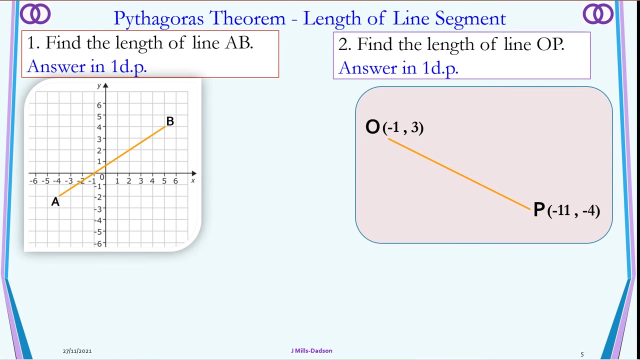 point eight squared minus five point two square. use a calculator, press the square button. it's square root button, first before 9.8 squared, then minus 5.2 squared, equal sign. then you approximate accordingly. sometimes you may be asked to find the length of a line segment. so examples like: 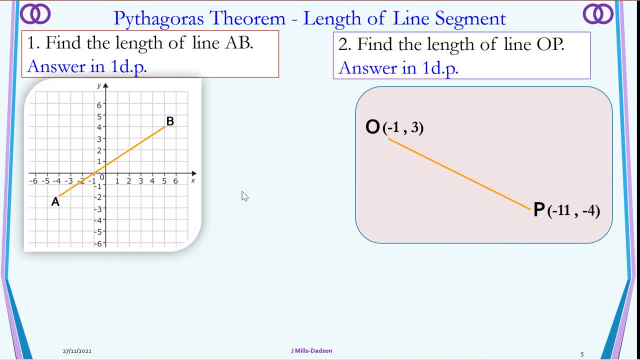 this. you could either be just a straight line with the coordinates given or just a line on a grade. they are all the same. so first here, work out your coordinates. so coordinate a is negative, 4, negative, 2, coordinate b is 5 and 4. and note your x and y coordinate. make a right angle triangle. 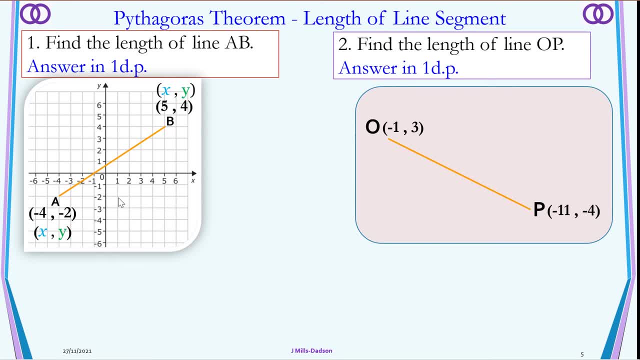 to connect a- b. so it could be this way or it could be the other way. whichever way doesn't matter. now what is left is to work out the length of the vertical line in the horizontal line. to work out the vertical line, you look at the gap between the y coordinates. 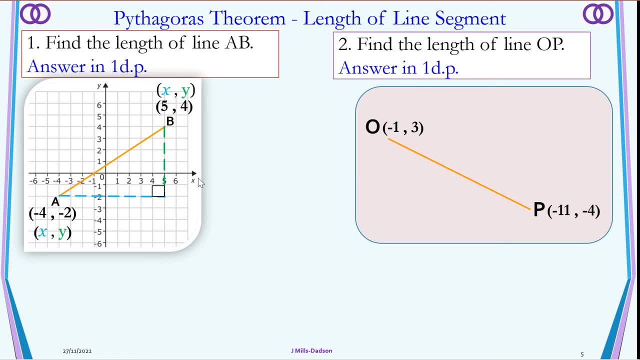 horizontal line. look at the gap between the x coordinates. so let's look at the vertical line. check the y coordinate. from negative two to four, count negative two to four. so negative one, zero, one, two, three, four, six steps. some people would like to do four minus minus two. 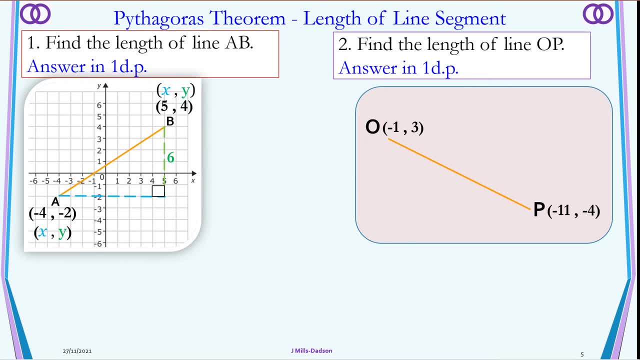 which will give you six. if you don't want to get into the complication, just count horizontal line. we are looking for the gap between negative four to five. so from negative four to five, count negative three, negative two and so on. you will know that the gap will be nine steps. 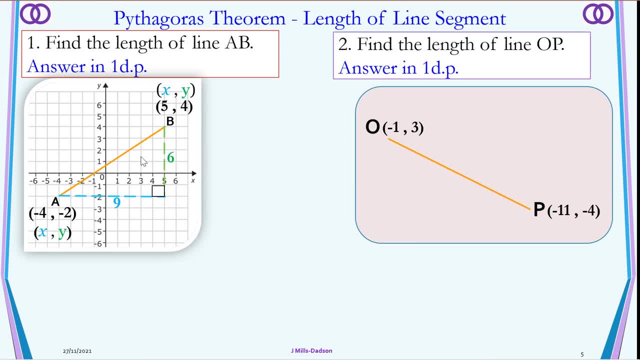 then you have a simple Pythagoras question: right angle triangle. obviously this will always become the longest side. so this kind of question for line segment is always the addition rule. it's always addition rule. so square root first and square each number, add them, find the square root. 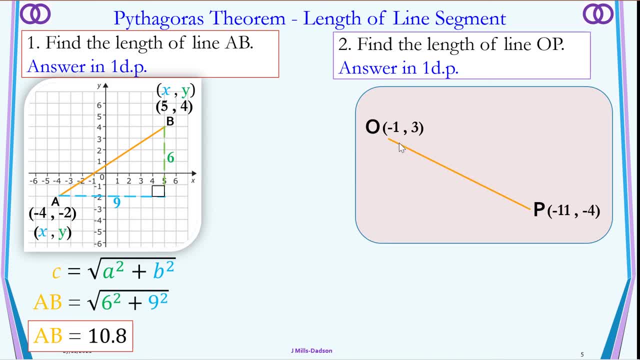 that's 10.8. second one: the same right angle triangle. you draw a right angle triangle gap between the y from three to negative four, from negative four to three. if you count you will know it's seven steps to 11. negative 11 or negative 11 to 1. if you count you see it's 10 steps hypotenuse. 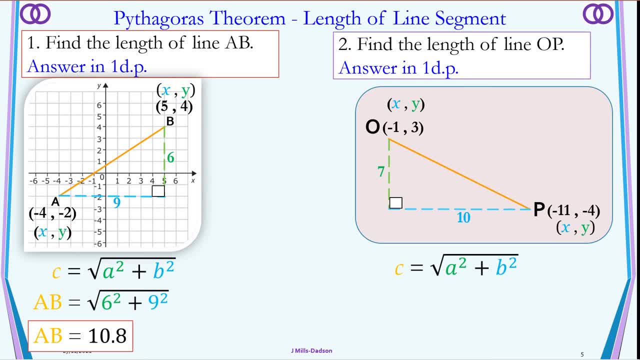 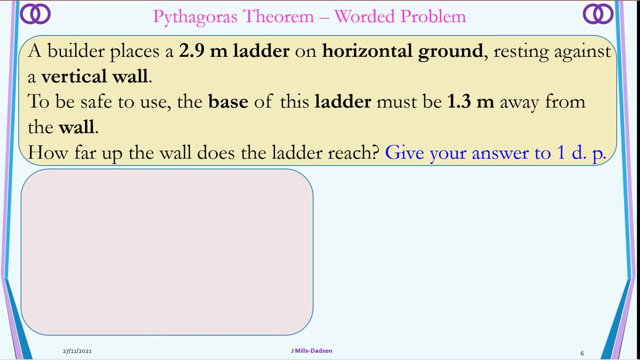 so it's addition rule: 10 squared plus 7 squared. find the square root of that quickly. that'll give you 12.2. so that is how we use it to work our line segment. now let's look at an exam style question. a builder places 2.9 meter ladder on a horizontal ground, resting against a vertical wall. 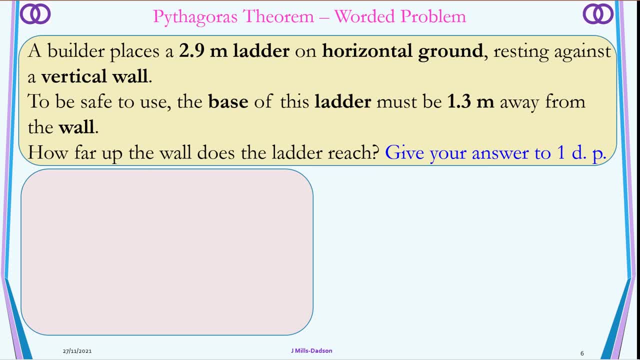 to be safe to use, the base of this ladder must be 1.3 meters away from the wall. how far up the wall does the ladder reach? give your answer to one decimal place. this kind of question, you need to use diagram to represent it for you to understand what you're supposed to do. so this is the ground. 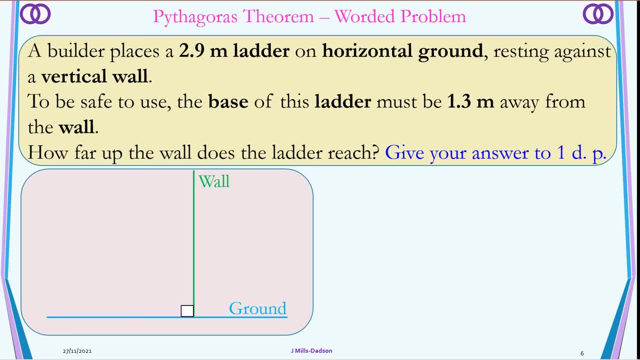 level ground. this is the wall. the wall is different: the upright, so vertical. now we've got the ground and the wall, we have our ladder. so this is the ladder. that's the first thing you need to know. now let's put in some numbers. it says the builder place: 2.9 meter. 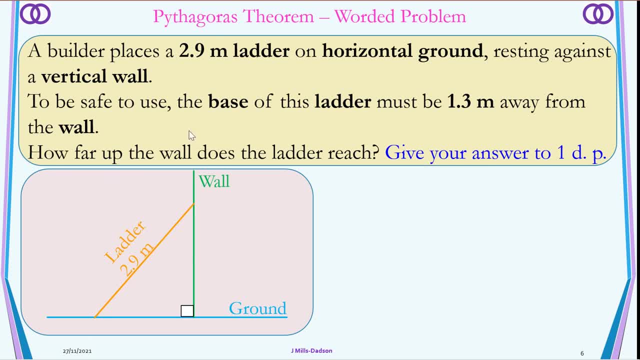 ladder on horizontal ground. okay, so 2.9 meter ladder, that's 2.9 rest on the vertical wall. okay, there's the wall. to be safe, the base of the ladder- this is the base of the ladder- must be 1.3 meter away from the wall. so this is the wall, this is the ladder, the gap between the 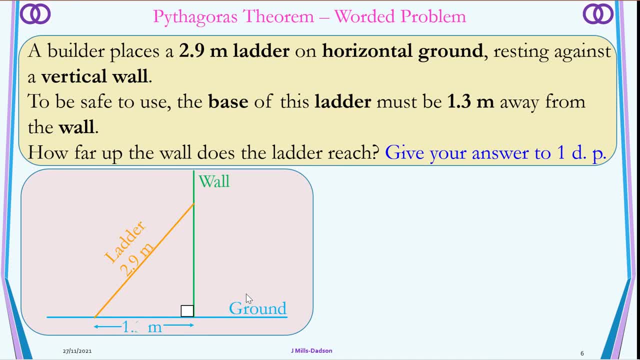 foot of the ladder or the base and the wall must be 1.3. how far up the wall does the ladder reach? the ladder reaches this height. so you want to see the length from the bottom here to this point. so it's still pythagoras. we check, it's not the longest side.